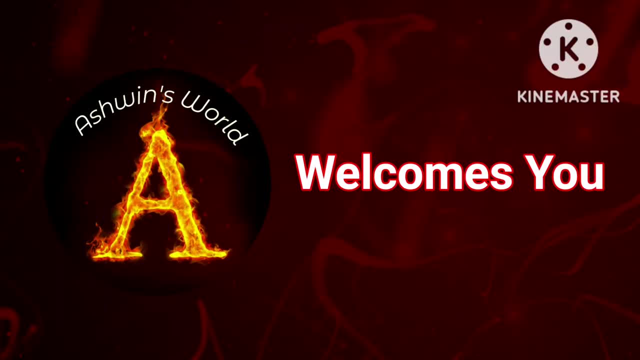 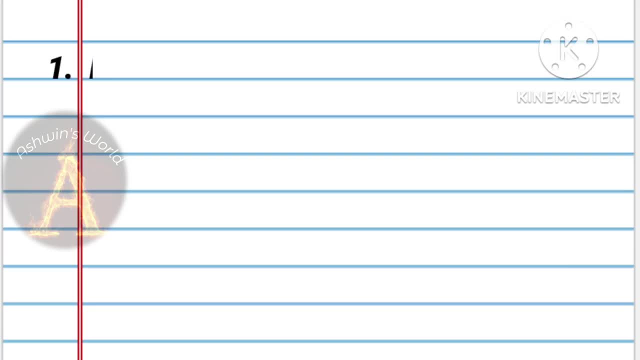 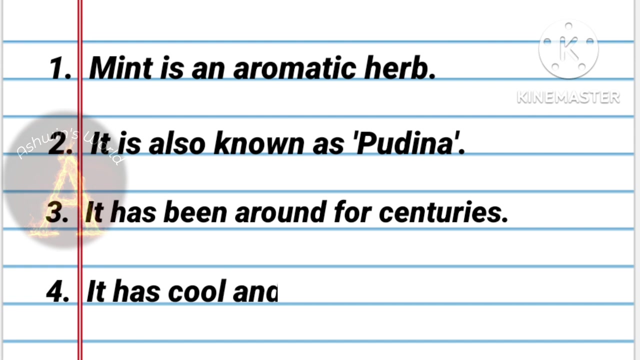 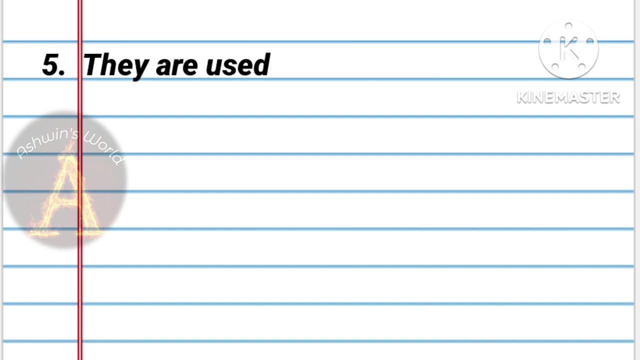 Hi friends, welcome to Ashwin's World. Ten lines on mint leaves. Mint is an aromatic herb. It is also known as Pudina. It has been around for centuries. It has cool and refreshing taste. They are used to add flavor to food and drinks. 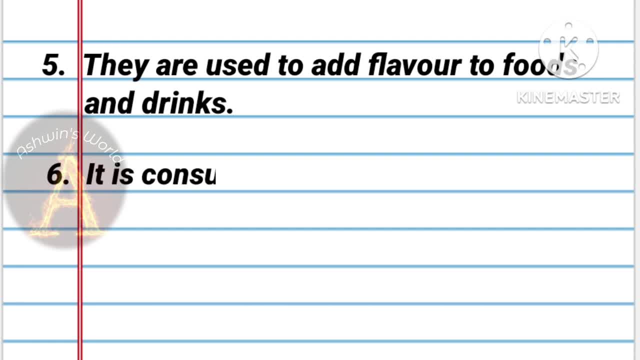 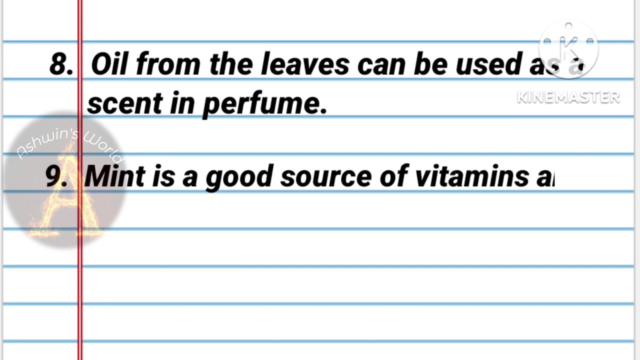 It is consumed as fresh or dried. The refreshing flavor can be used in candy and toothpaste. Oil from the leaves can be used to make a drink. It is also used as a scent in perfume. Mint is a good source of vitamins and antioxidants. 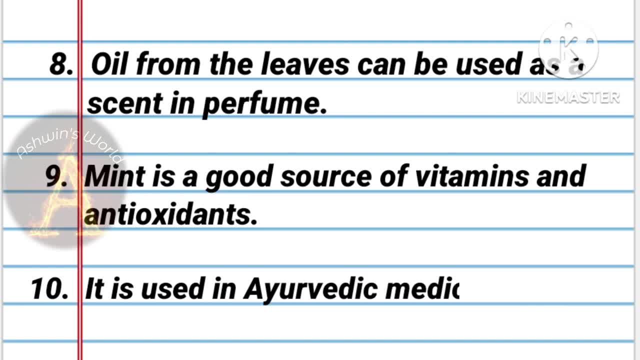 It is a great source of glycolic. anti-inflammatory, anti-inflammatory, anti-inflammatory, anti-inflammatory, anti-inflammatory. It is a very healthy plant that can be used as a food supplement. Mint is a healthy plant that is rich in fiber, vitamin C and a good source of vitamin A.